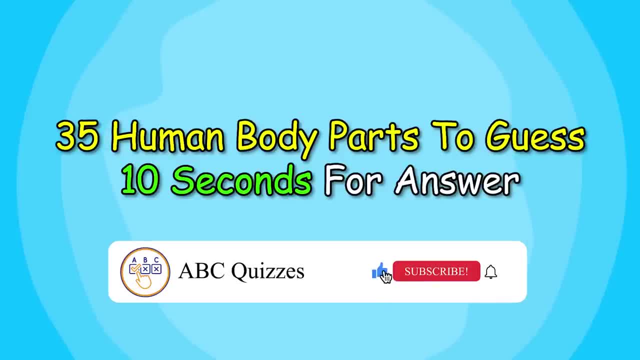 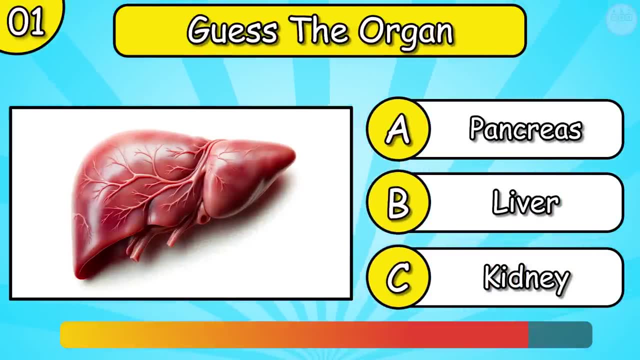 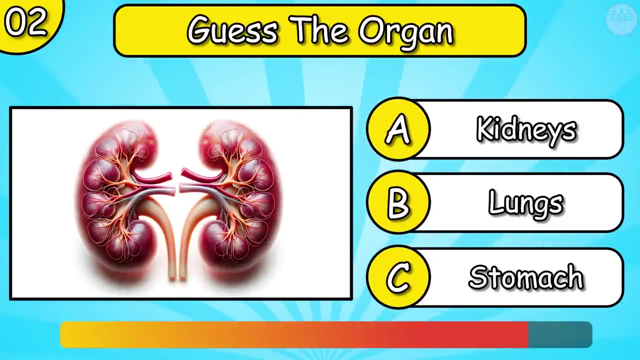 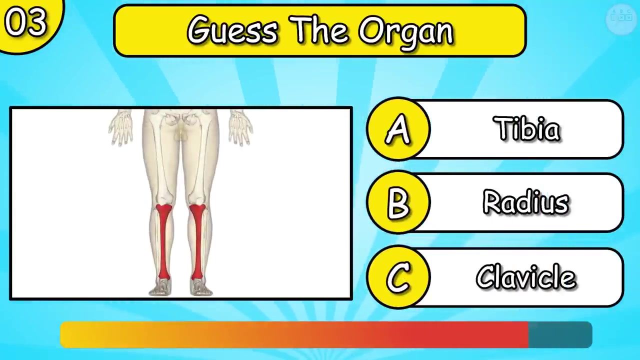 Hello ABC Quizzers. In today's quiz you'll have to guess 35 human body parts. You will have 10 seconds for an answer. Let's start. Guess the organ: It's liver, It's kidneys, It's tibia. 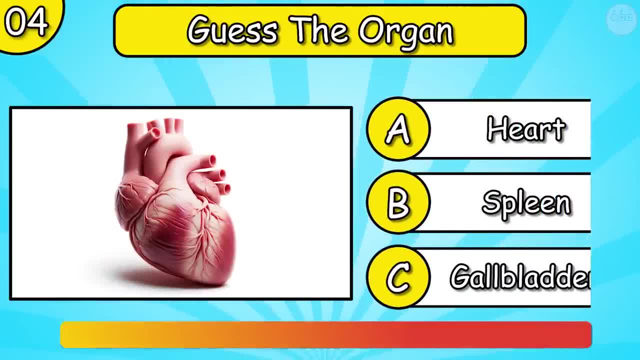 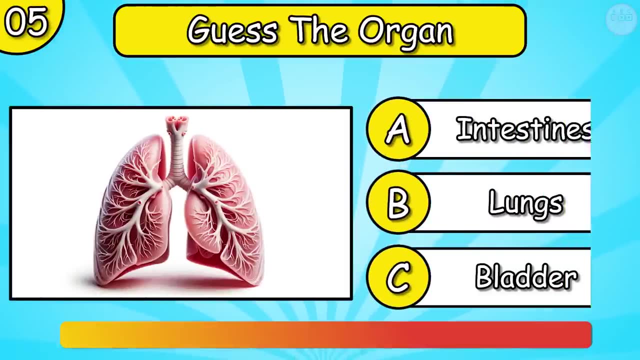 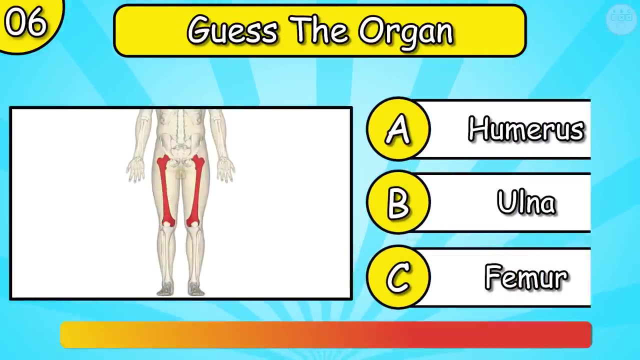 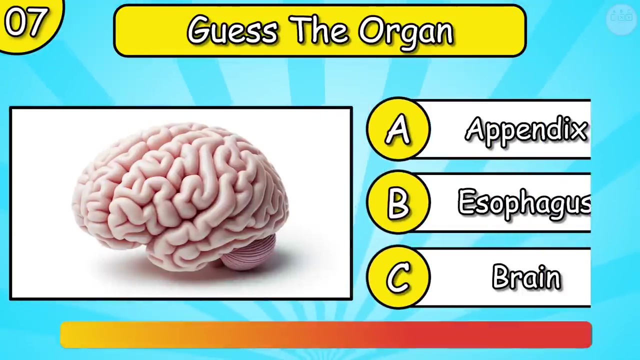 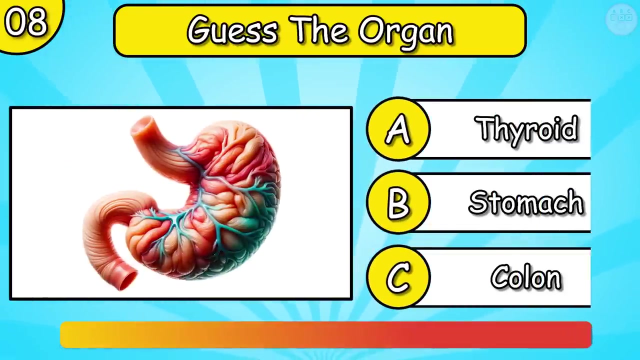 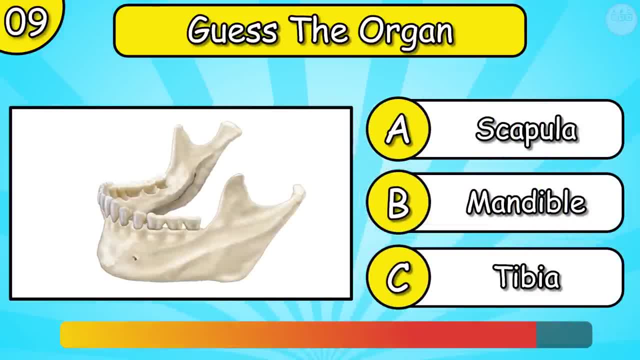 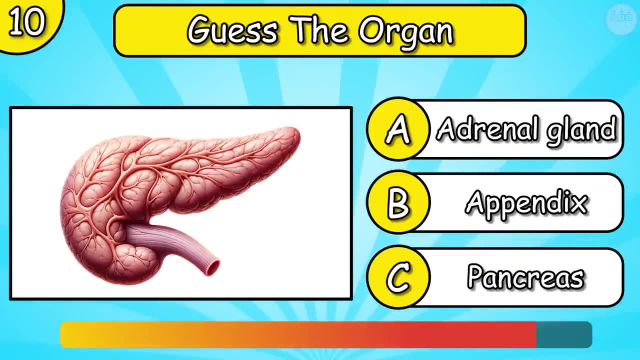 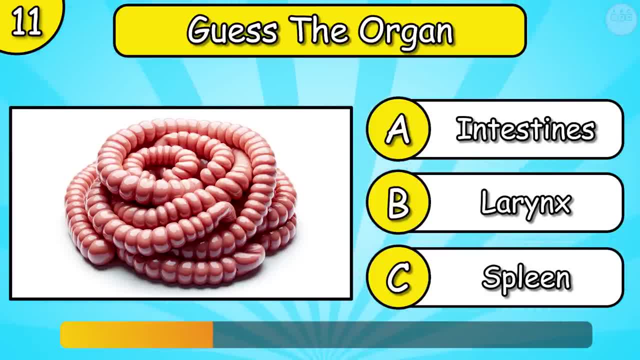 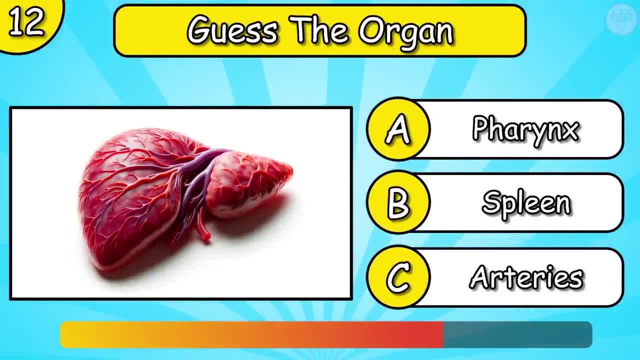 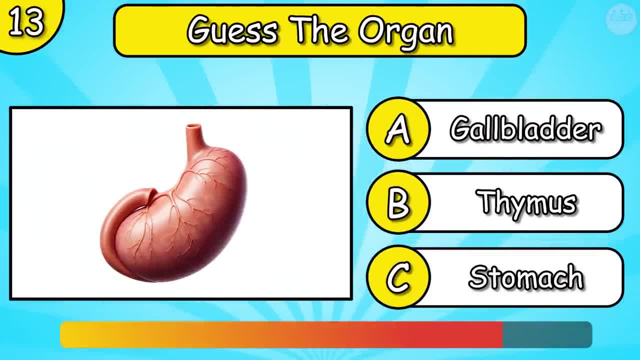 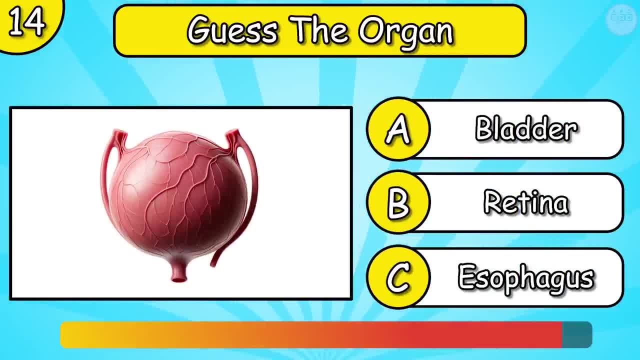 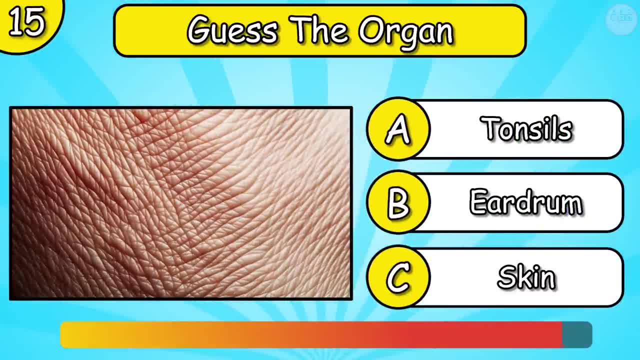 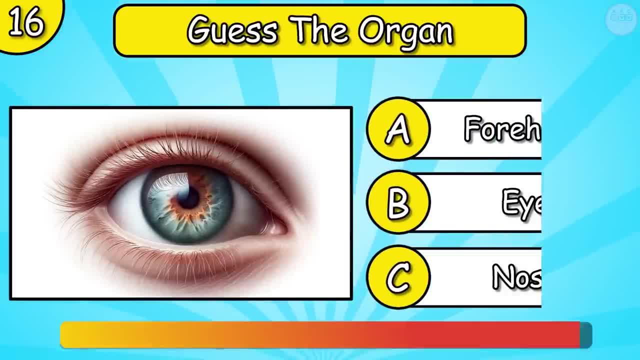 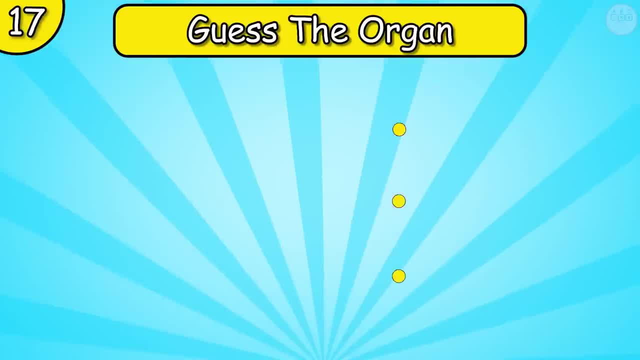 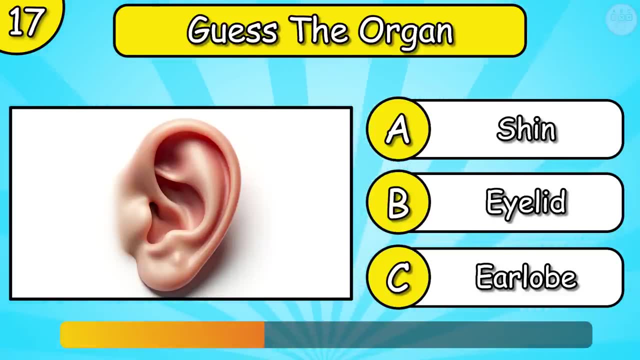 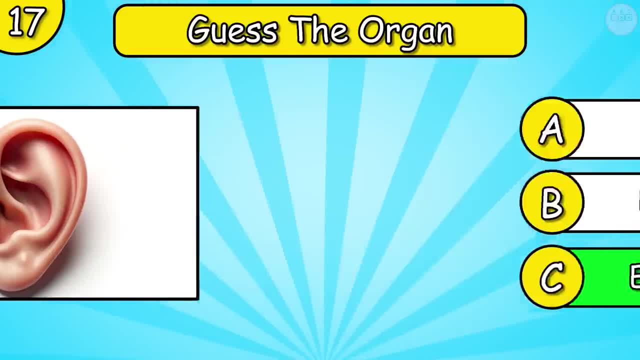 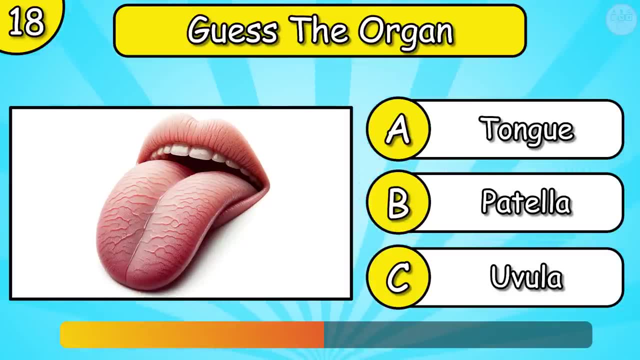 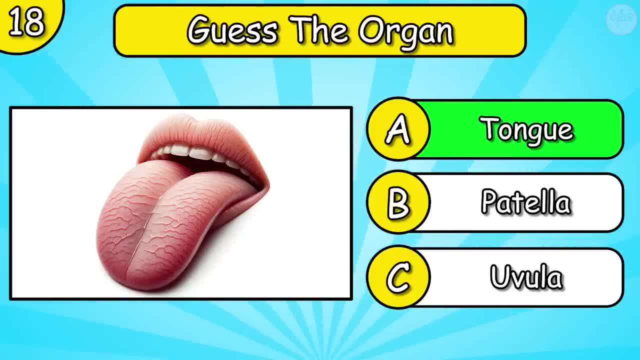 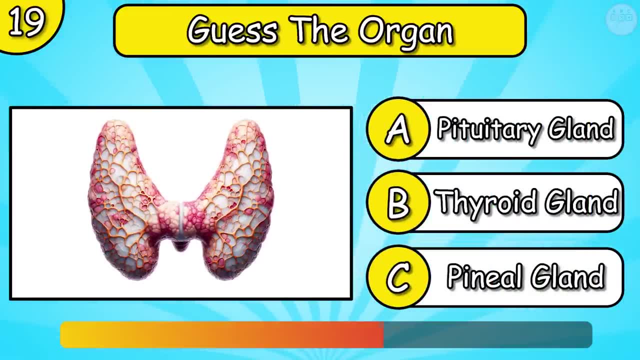 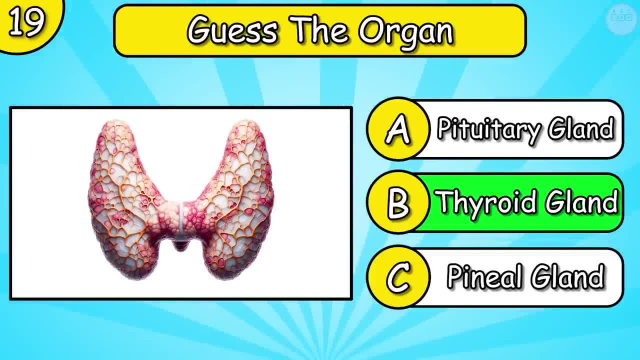 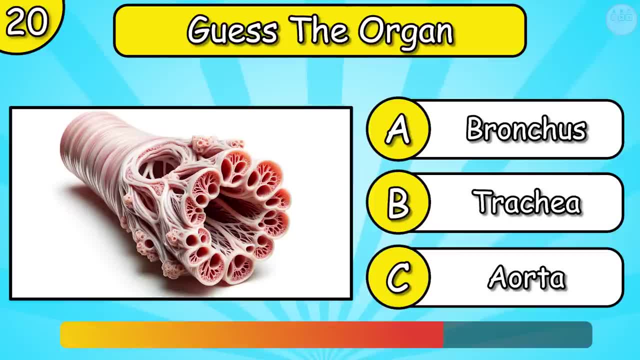 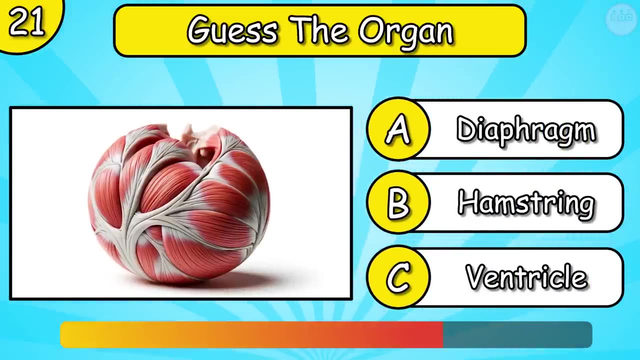 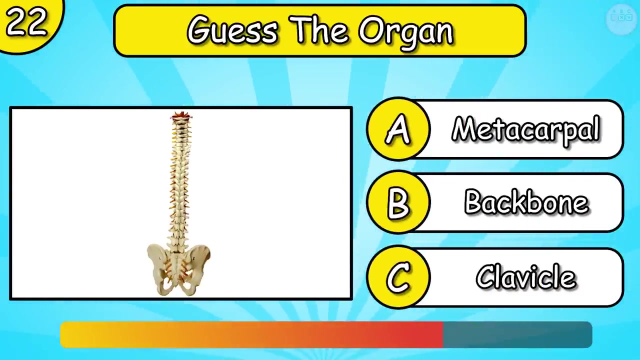 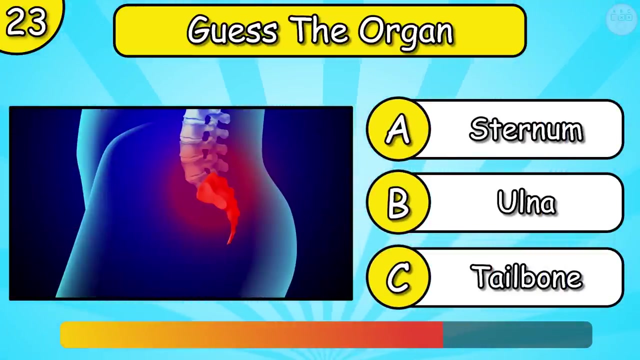 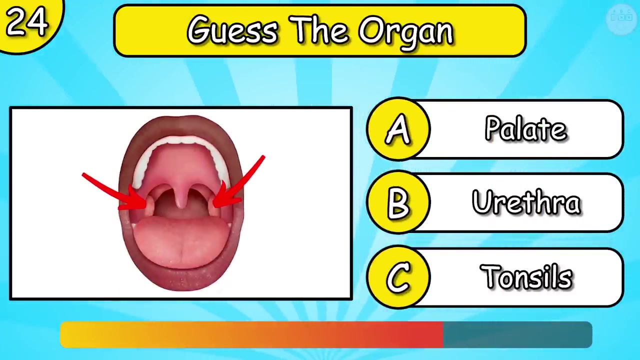 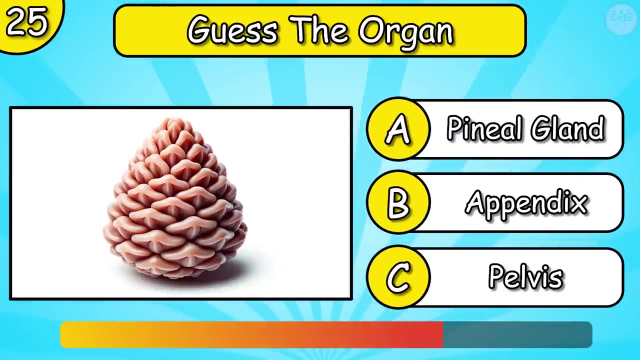 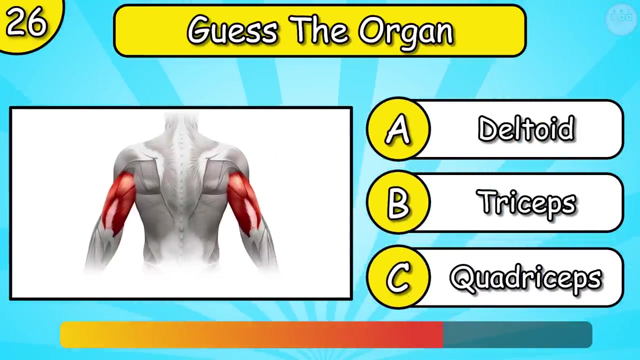 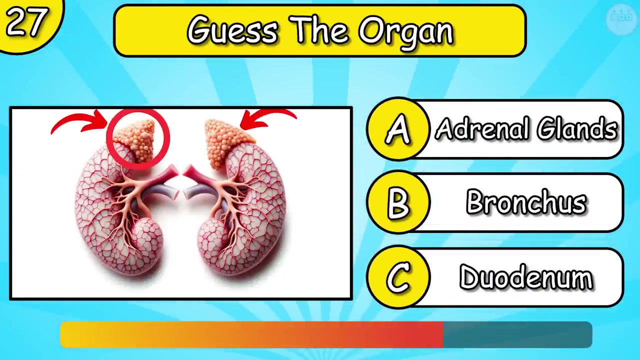 Pancreas, Pancreas, Pancreas, Pancreas, glans, Trachea, Diaphragm, Backbone, Tailbone, Tonsils, Pineal gland Triceps. Adrenal glands gold, Tash, Trixie, Tats, Trixie, Trixie.